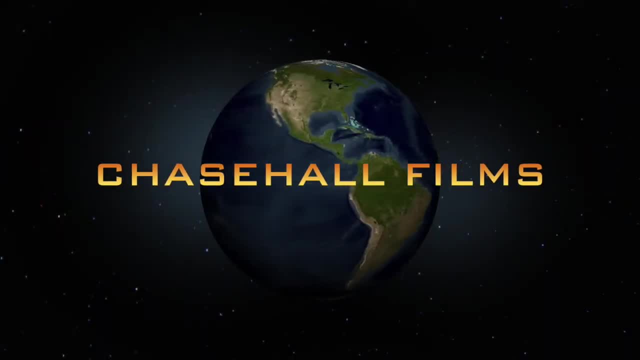 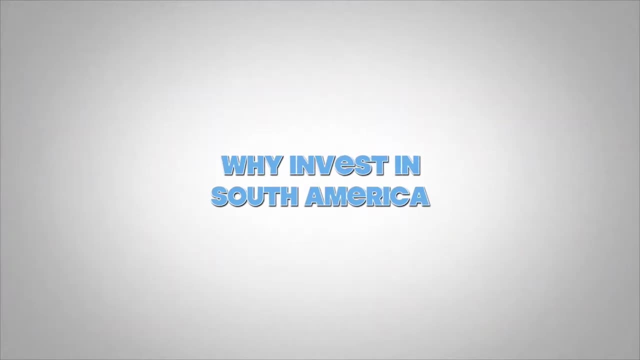 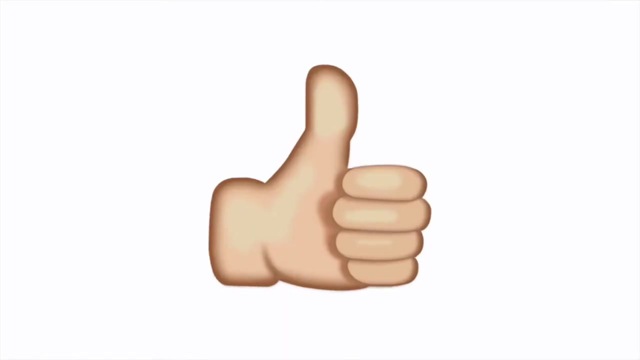 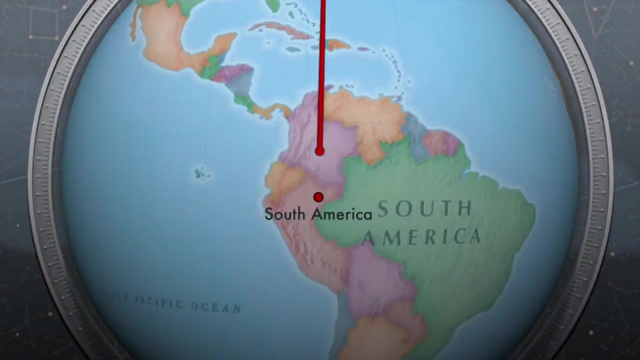 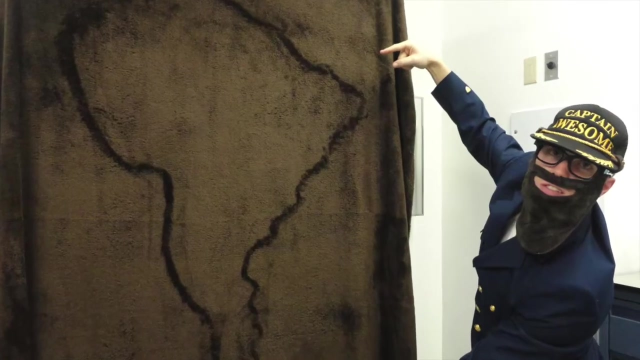 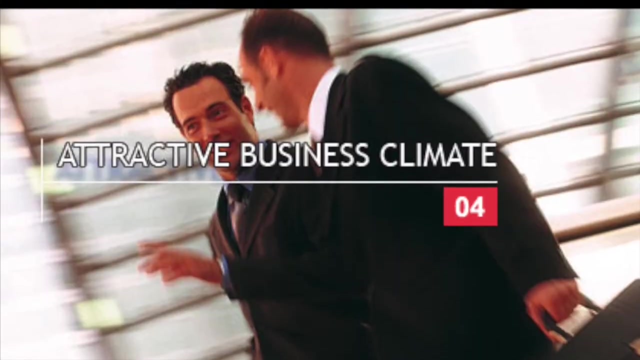 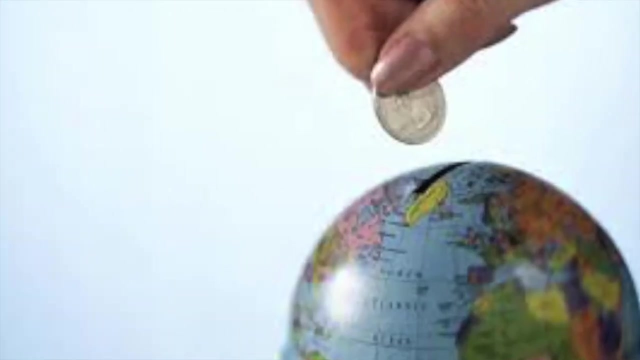 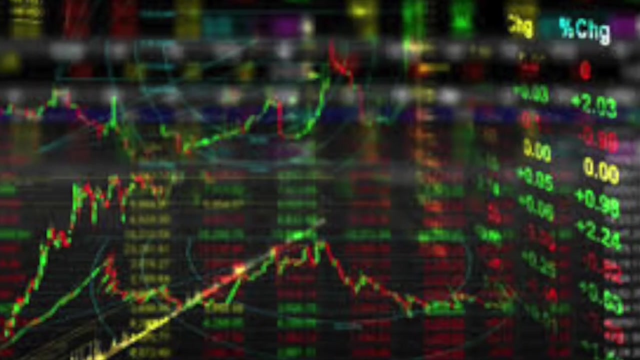 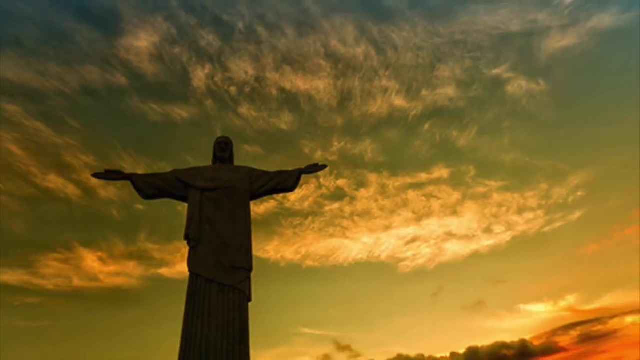 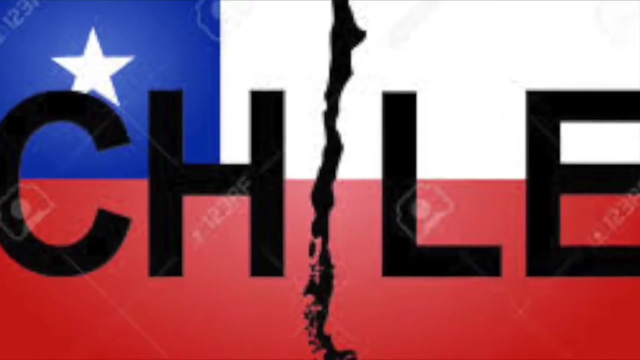 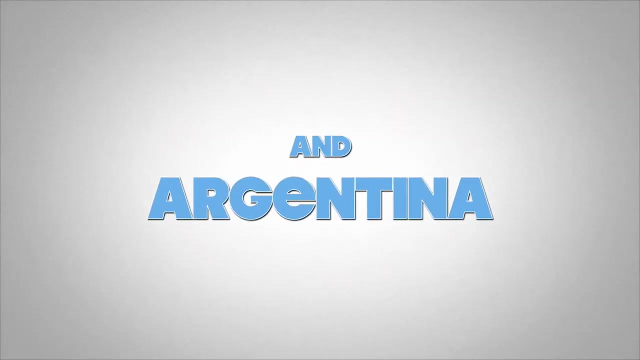 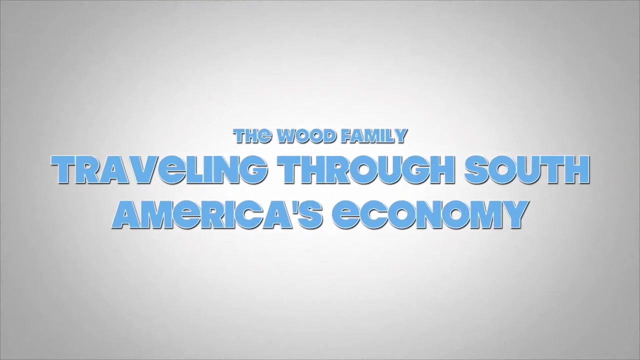 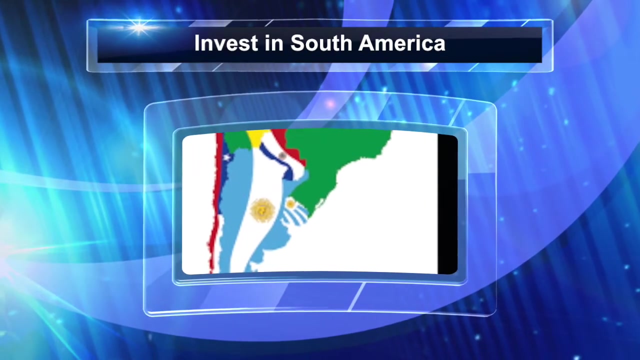 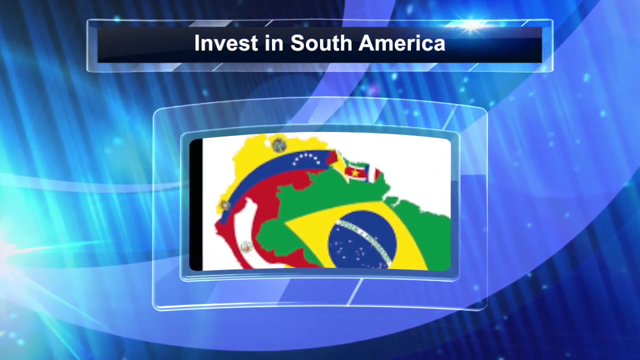 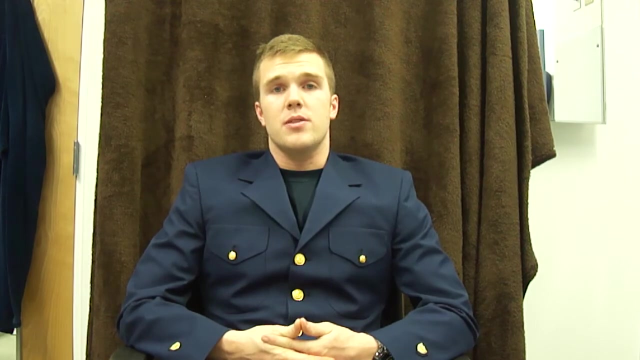 Thank you for watching. Thank you for watching. Thank you for watching. Hello and welcome to Macro Talk. Today we will be discussing the economy of South America. We will be focusing on five countries that are the best indicators of the economy of South America as a whole. 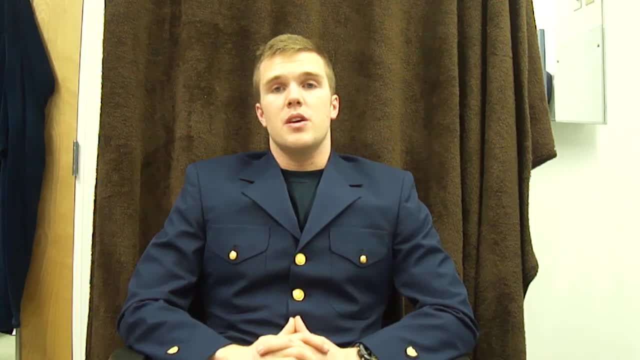 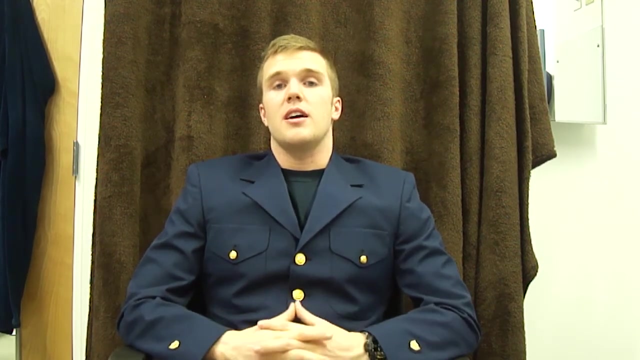 Argentina, Brazil, Chile, Colombia and Peru. In each of these countries, economies will focus on five major investment indicators: GDP, annual GDP growth rate, unemployment rate, interest rate and inflation rate. An analysis of these indicators in each of these five countries will give you the best idea of why South America is the place to invest. 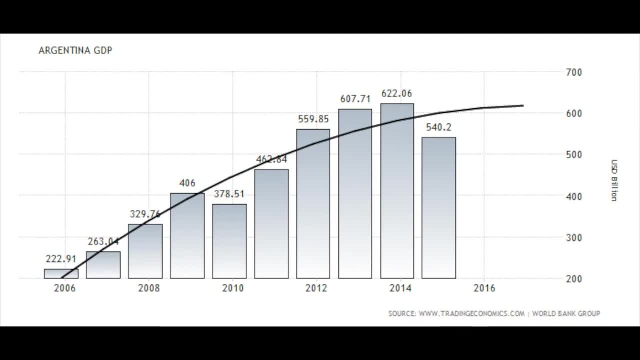 Argentina is one of South America's largest economies, Endowed with rich natural resources. the country also benefits from a well-educated workforce, an expert-oriented agriculture sector and a diversified industrial base, Although the agricultural sector represents less than 10% of the GDP. 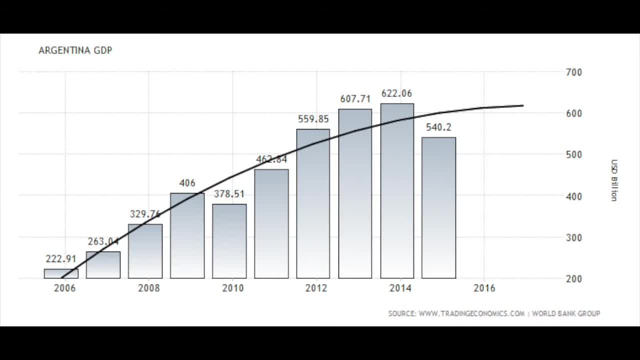 Argentina is one of the world's largest exporters of soybeans, wheat and meat. The services sector accounts for over 60% of the GDP, supported by a girding number of financial and tourism enterprises. The industrial sector accounts for around 30% of GDP. 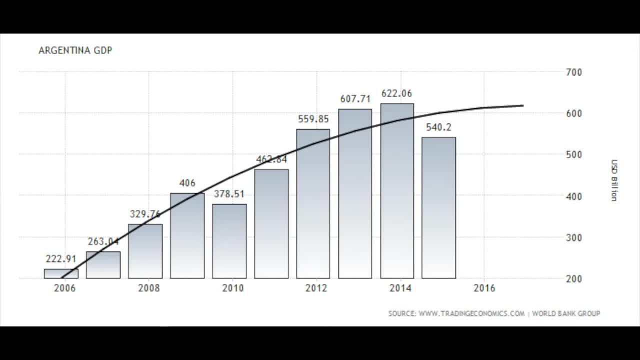 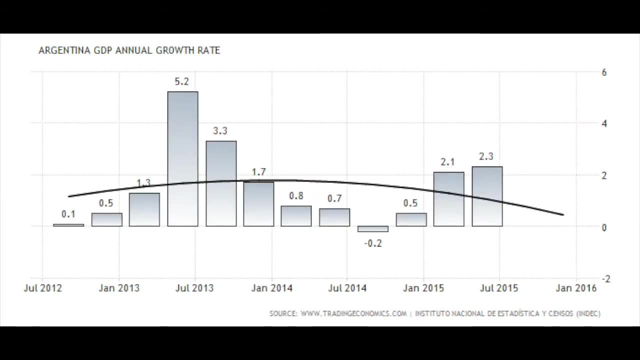 including food processing, oil refining machinery and equipment, textiles, chemicals and proto-chemicals. The GDP in December 2014 was $540 billion. The GDP annual growth rate is growing 2.3% each year. This is good for investors because each year, Argentina is making more and more and increasing the standard of living of life. 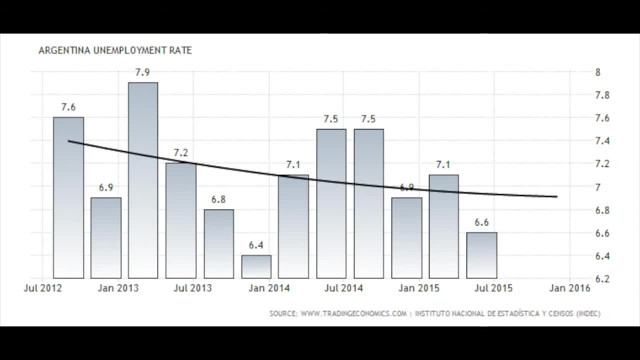 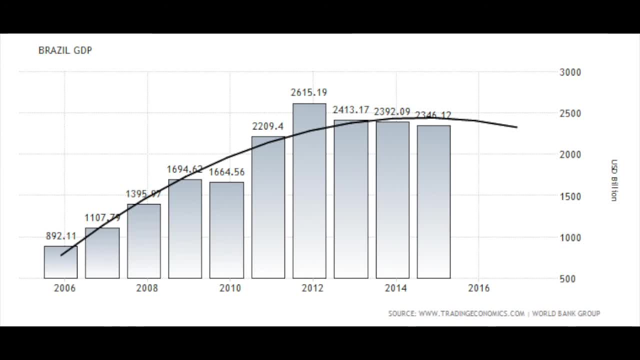 this represents the majority of Argentinians are working and million head. other important agricultural products include soybeans, corn, cotton, cocoa, tobacco and forest products. industry accounts for one-third of gdp, with well diversified sectors ranging from automobiles, machinery and equipment, steel, textiles, cement, petrochemicals and consumer durables. 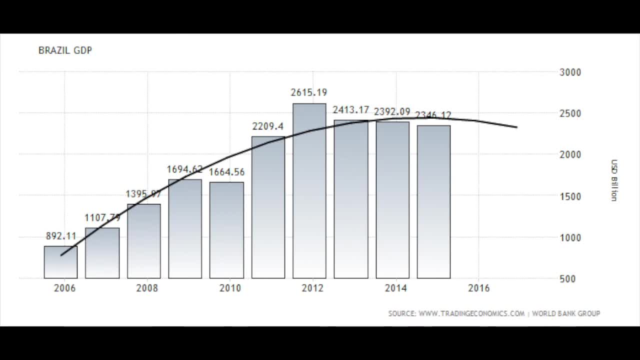 contributing about 65 to gdp. brazil's service sector is diverse and sophisticated, including telecommunications, banking, commerce and computing. brazil also has the largest rainforest in the world, located in the amazon basin, and is one of the world's leading producers of hydroelectric power. over the past decade, brazil has built a strong macroeconomic framework. 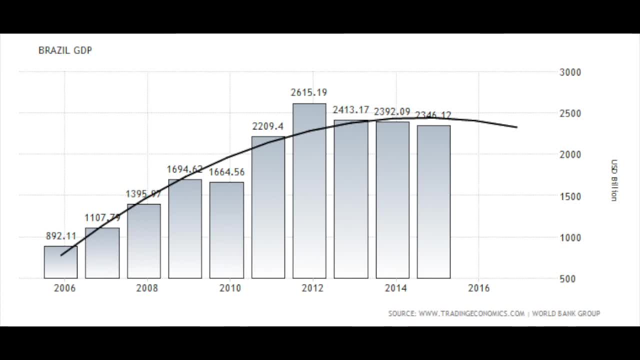 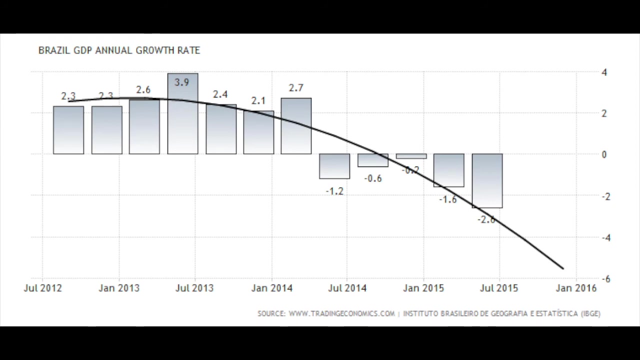 including fiscal discipline, inflation targeting and the flexible exchange rate regime. while burning reforms and prudent macro macroeconomic policies, the government has also moved to narrow gaps between the rich and the poor. gdp in december of 2014 was 2 346 billion dollars. the gdp annual growth rate, however, is decreasing at a rate of 2.6 percent a year, which unfortunately 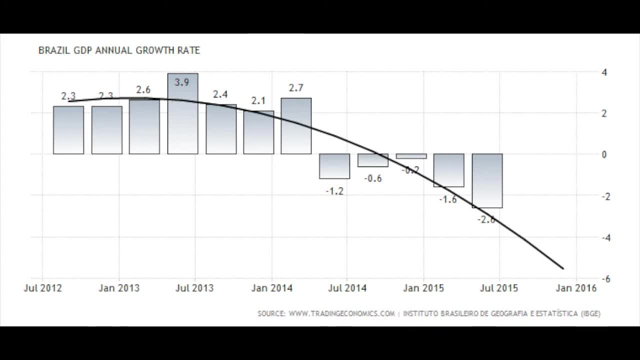 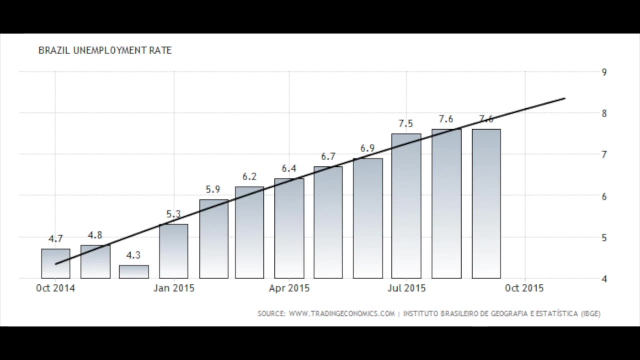 is not that exciting for investors. however, with the olympics coming up, the possibility for that gdp to spike is increasing rapidly. the unemployment rate, however, is um is 7.6 and it's very stable, so that's very attractive to investors. the inflation rate is at 9.49, which 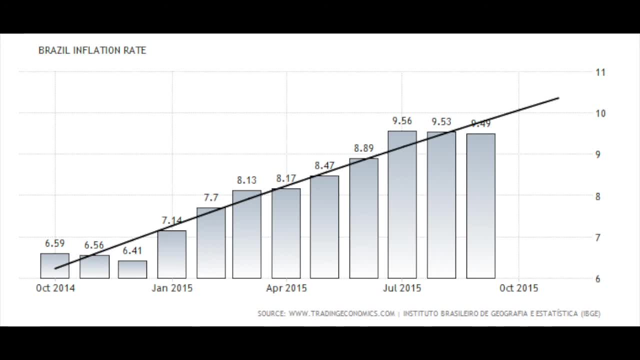 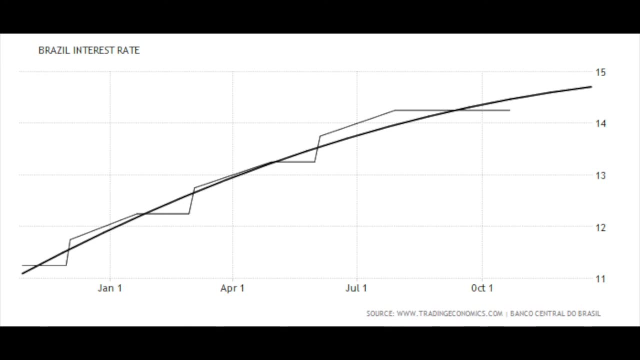 indicates that the government is trying to pump money back into the economy to help stimulate growth even more. the interest rate is currently at 14.25 percent and trending upwards, which is very attractive to foreign investors. as we see as the interest rate rises, we see an increase. 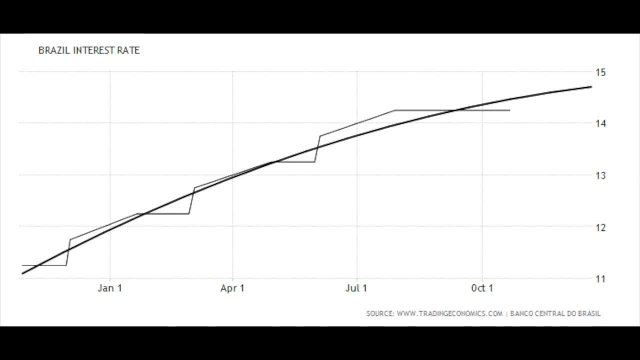 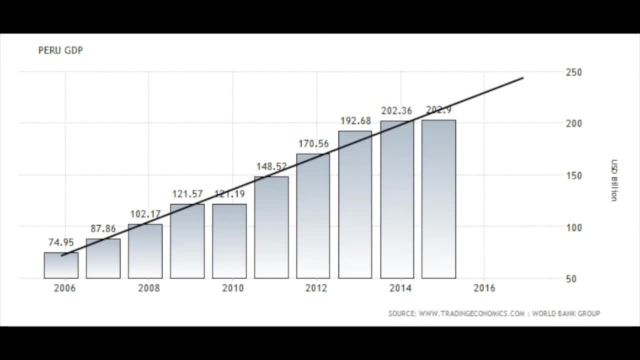 in the viability of foreign investment. in reality, peru is like the nucleus of the cell. it has mineral resources and excellent fishing. there's nothing else you need in the economy. as you look at the gdp, the gdp of peru is at a staggering 202.9 billion dollars. the gdp may not be the highest number out there, but we're going for. 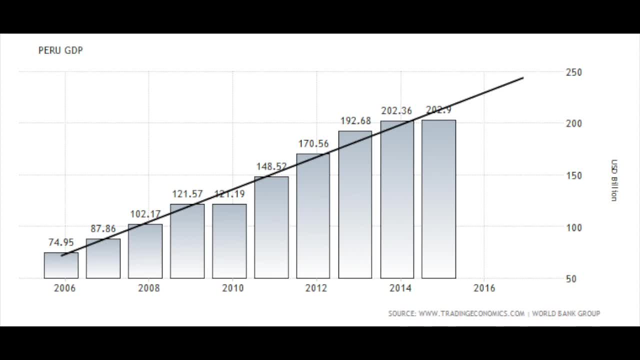 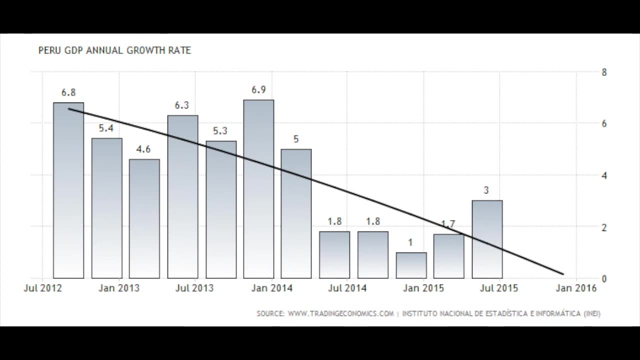 quality over quantity in south america. peru is at a staggering 202.9 billion dollars. peru is at a staggering 202.9 billion dollars. In Peru currently the GDP annual growth rate is decreasing, but that is not stopping the actual GDP from increasing, apparently. 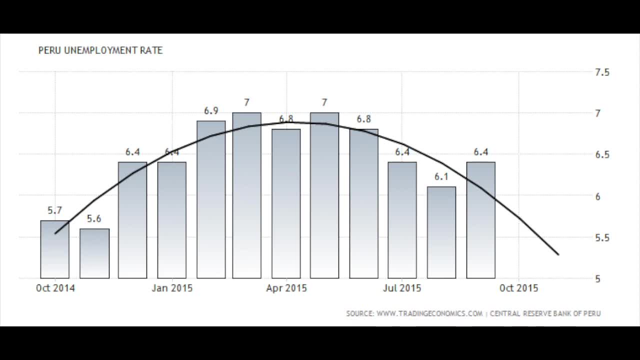 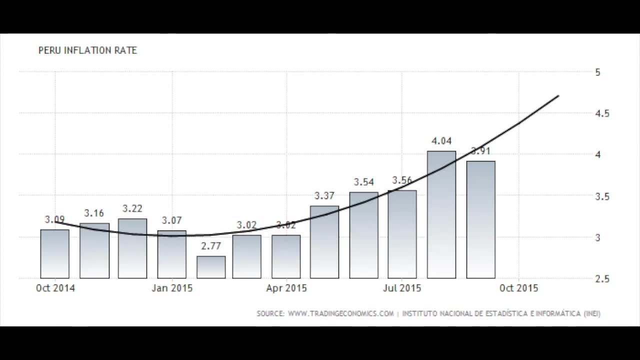 The unemployment rate is at a stable 6.4%, and let me repeat, 6.4%. The inflation rate is on the upward rise, but in the last year it did decrease, so that could be the start of a downward trend in inflation.